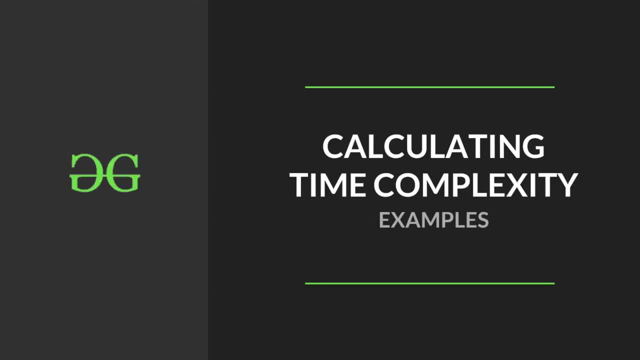 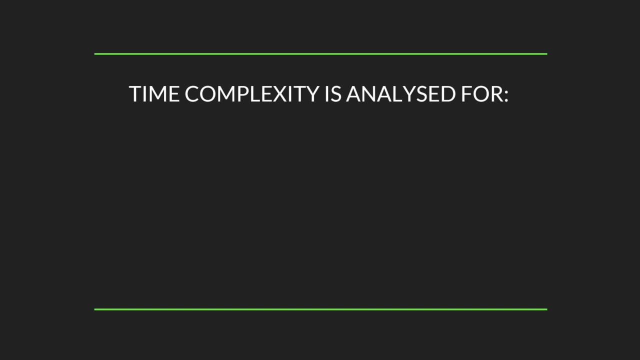 Hello friends, And welcome to this video in which we will learn about some of the techniques using which we can easily calculate time complexity of algorithms without complex calculations. So let's get started. One thing to be noted is that time complexity is analyzed for very large input size and 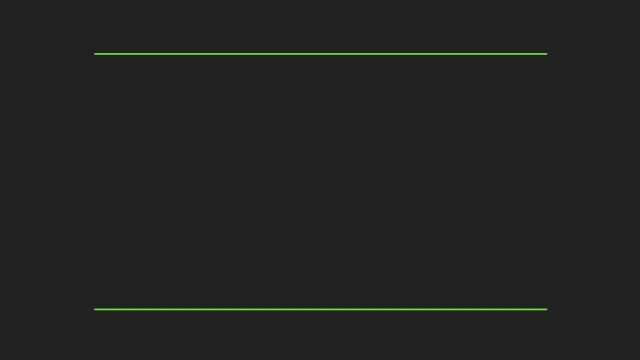 worst case scenarios. Now let's take an example and try to calculate its time complexity. So we have tn, which is equal to 2n square plus 3n plus 1.. The first step is to drop the lower order terms, that are 3n plus 1 in. 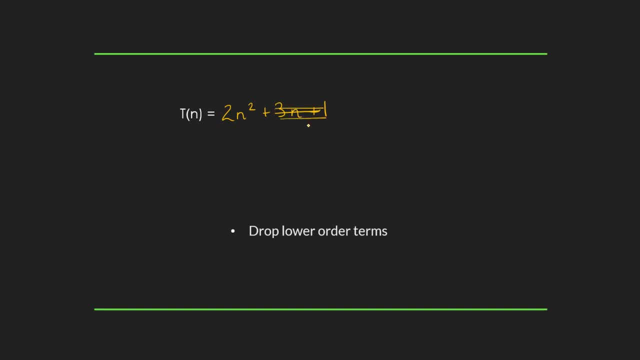 this case. Next, we drop the constant, that is 2.. So we get the time complexity as O for this particular polynomial. Now let's look at some rules for finding out the time complexity in algorithms. First let us look at how do we calculate the time complexity of a single loop. 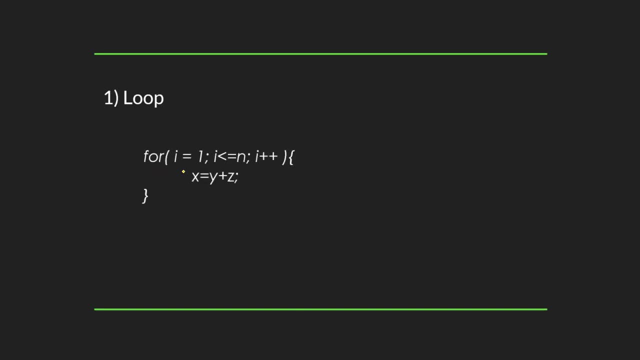 So this is our for loop, which runs from 1 to n, And we have this expression inside the for loop, x equal to y plus z, which takes constant time to execute. Now the time complexity will be n times time taken for this expression, which is a constant. 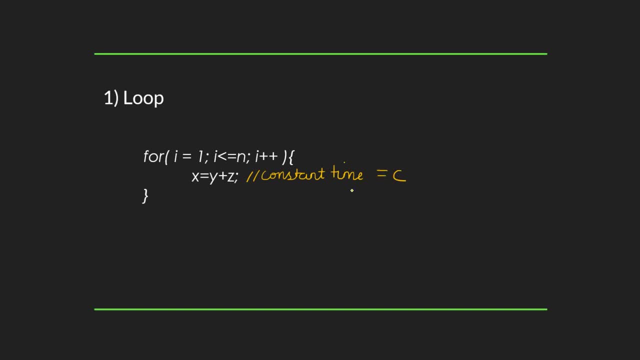 let's say c, So the time complexity will come out to be c times n And in O terms we can neglect this constant and simply write the time complexity as O of n. Now let's look at nested loops. As you can see, we have two loops which are: 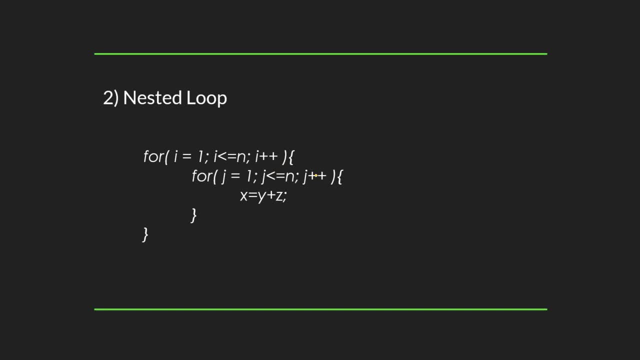 nested. Let's try to find out the time complexity. So this is the expression which takes constant time to execute. Now we simply multiply the time complexity of each loop. So this is the outer loop, which will run n times. And for each run of the outer loop, this inner loop will also run n times. 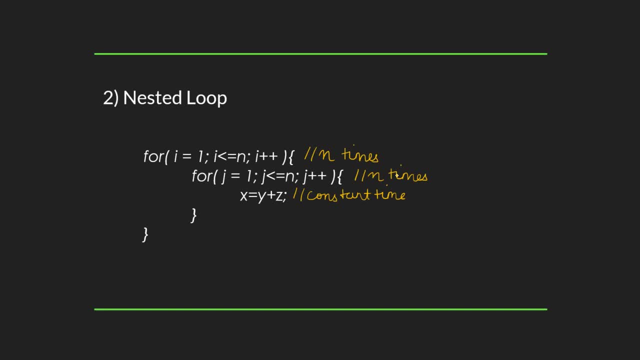 So the time complexity of the inner loop will also run n times. So the total running time will be some constant time multiplied by n into n, which is equal to n square. So we can say that the time complexity is O of n square. 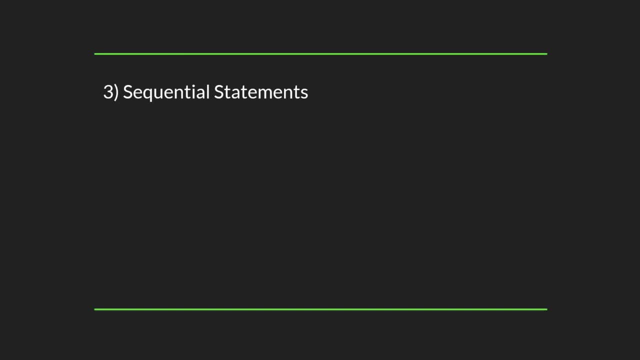 Next are the sequential statements. Let's say that we have an expression which takes constant time to run. Let me denote it by a constant time. So we can say that we have an expression which takes constant time to run. Let me denote it by a constant time. 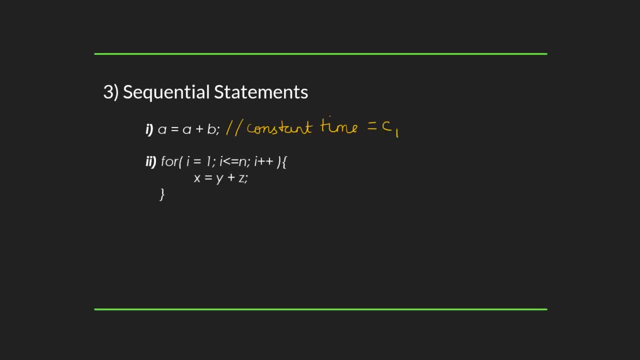 After that we have this fall loop which we have seen before, and it will take C2 times n time to run. Then we have another fall loop which takes C3 into n time to run. So when we have sequential statements like these, we simply add the time taken for each. 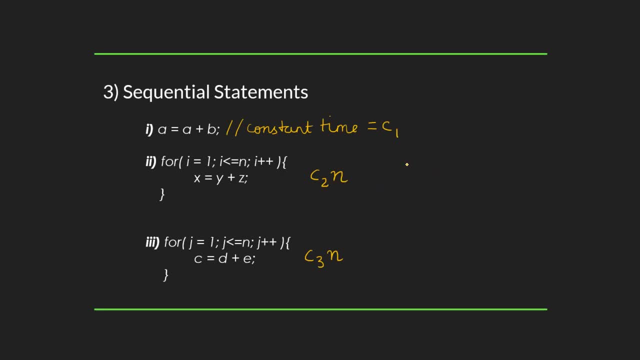 statement. So when we have sequential statements like these, we simply add the time taken for each statement. So let me do that In O terms. we can ignore these constants C1, C2 and C3 and we have the time complexity. 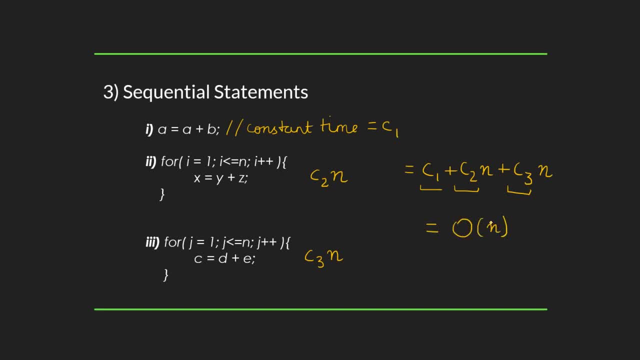 as O Next. let us look at how do we find out time complexity when we have conditional statements. For example, we can write the time complexity as O Next. let us look at how do we find out time complexity when we have conditional statements. 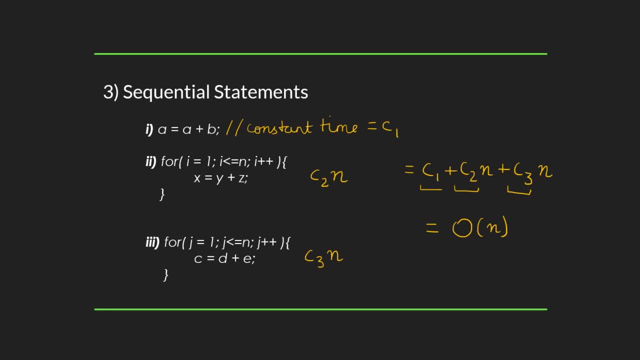 For example, we can write the time complexity when we have conditional statements. When we have conditional statements, such as if else, we evaluate the donation when values in if else conditions cause maximum number of statements to be executed. So let us say that inside this if condition, we have a fall loop whose time complexity 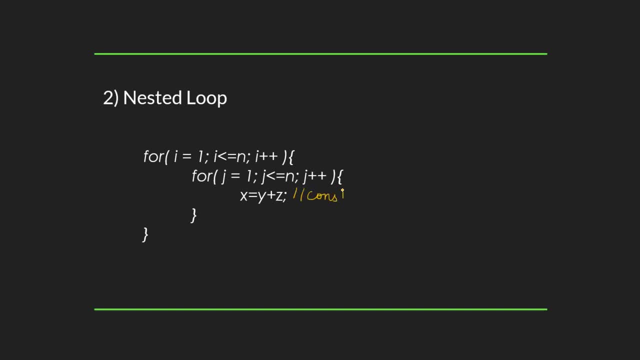 So this is the expression which takes constant time to execute. Now we simply multiply the time complexity of each loop, So this is the outer loop which will run n times, And for each run of the outer loop, this inner loop will also run n times. 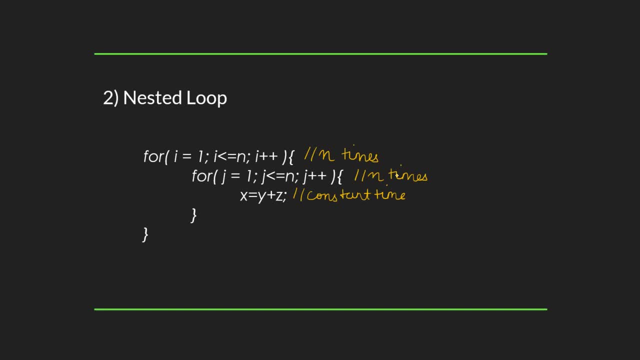 So the total running time will be: So the total running time will be: So the total running time will be Some constant time multiplied by n into n, which is equal to n square, So we can say that the time complexity is O. 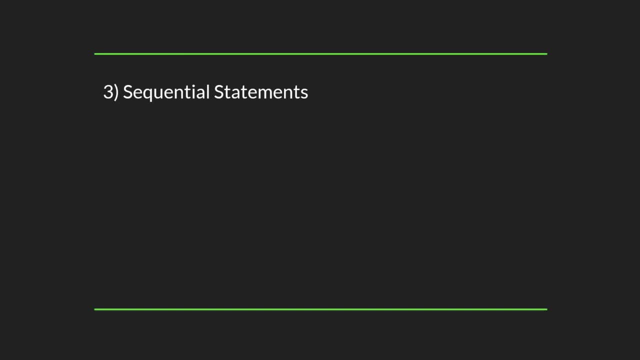 Next are the sequential statements. Let's say that we have an expression which takes constant time to run. Now let's say that we have an expression which takes constant time to run, denoted by c1.. After that, we have this for loop, which we have seen before, and it will. 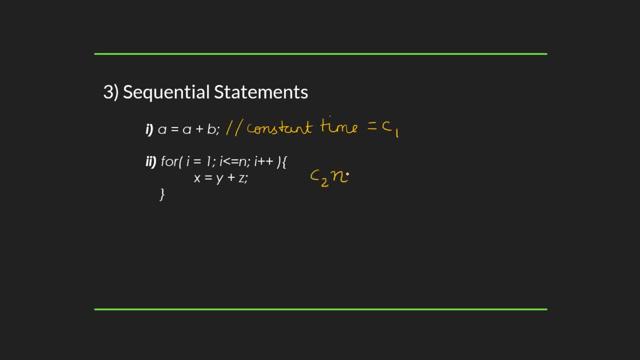 take c2 times n time to run. Then we have another for loop which takes c3 into n time to run. So when we have sequential statements like these, we simply add the time taken for each statement. So let me do that. 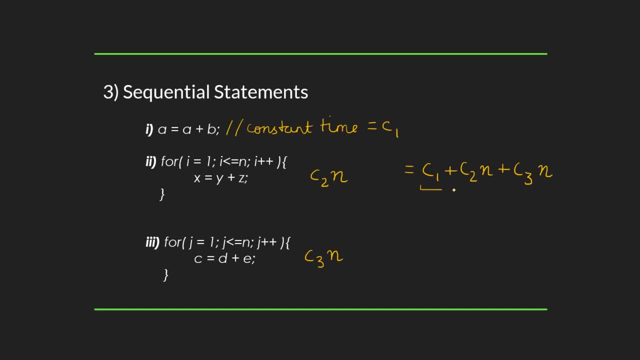 In O terms, we can ignore these constants c1, c2 and c3 and we have the time complexity as O. Next, let us look at how do we find out time complexity when we have conditional statements such as if-else. We evaluate the situation when values in if-else conditions cause maximum number of. 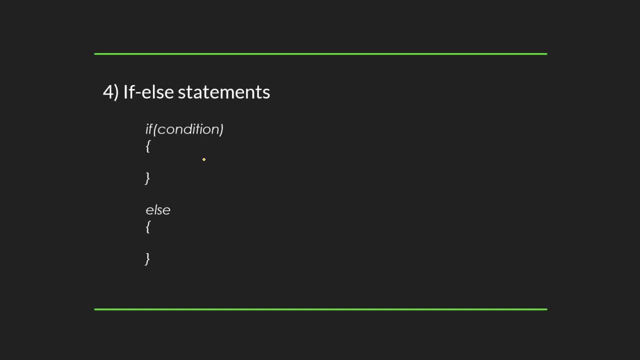 statements to be executed. So let's say that inside this if condition we have a for loop whose time complexity is O, And inside this else condition we have a nested for loop whose time complexity is Big, o. So we consider the else condition as it has. 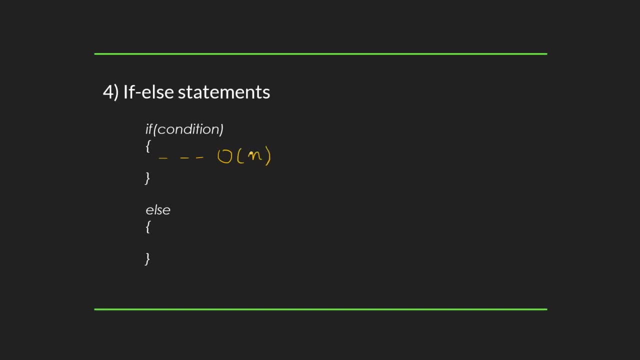 is big O And inside this else condition we have a acted NestedFallLoop whose Time Complexity is O O. So we consider the else condition as it has a greater time complexity And hence the overall time complexity will come out to be. 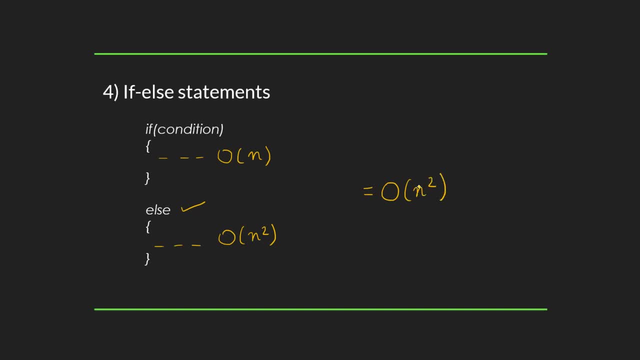 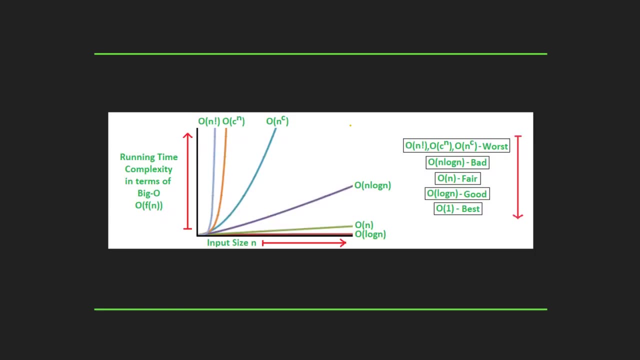 O. Now let's look at the comparison of time complexities. So we have O, which is the smallest and the best, Then we have O, Then comes O, Then it is O, Then we have O And finally we have O, which is the worst. 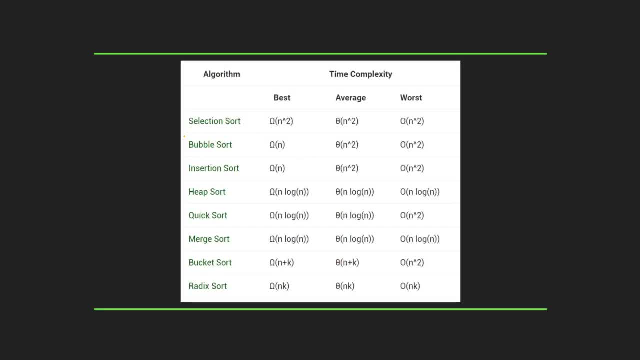 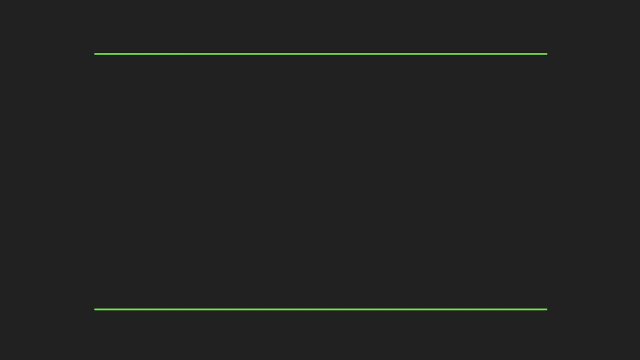 This is a chart of time complexity of various sorting algorithms. It is highly recommended to learn them by heart, as it comes very handy. Alright, So till now we have only talked about time complexity of a program. However, there is another factor which affects the execution. 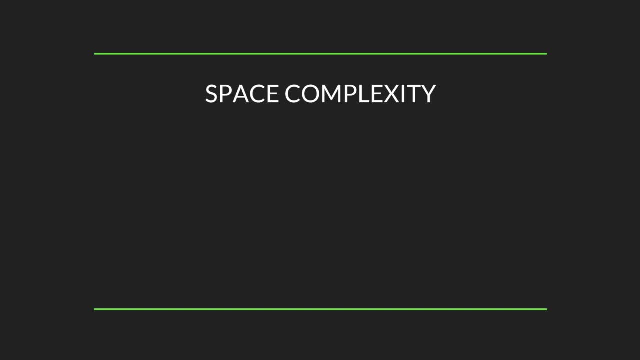 of a program which is space. Space complexity of an algorithm quantifies the amount of space or memory taken by an algorithm to run as a function of the length of input. Let's quickly understand it with an example. Assuming that an integer takes 4 bytes of. 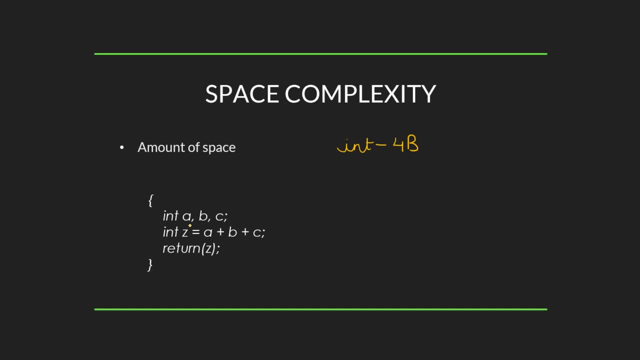 storage in memory. And in this piece of code we have 4 integers: a, b, c and z, So the total space will come out to be 4x4 plus 4.. This additional 4 is for the return statement. Hence this comes out to be 20 bytes. So 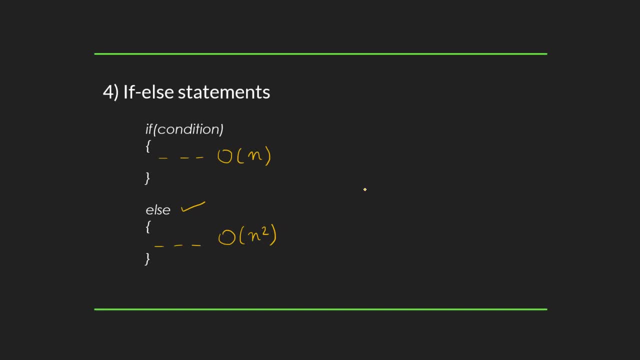 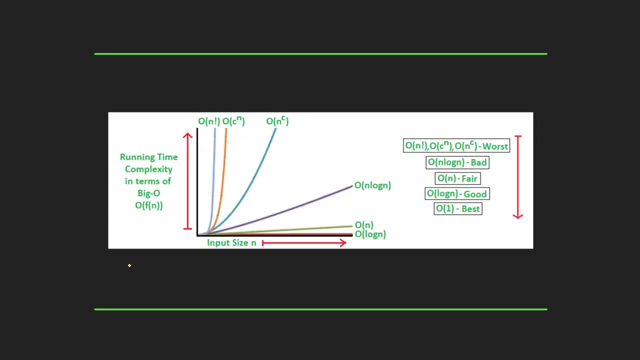 a greater time complexity and hence the overall time complexity, will come out to be O Sache. Now let's look at the comparison of time complexities. This is our case. Here's our而且 monitoring the time complexities. So we have Big o, which is the smaller term or such, and the base vectors of the other. 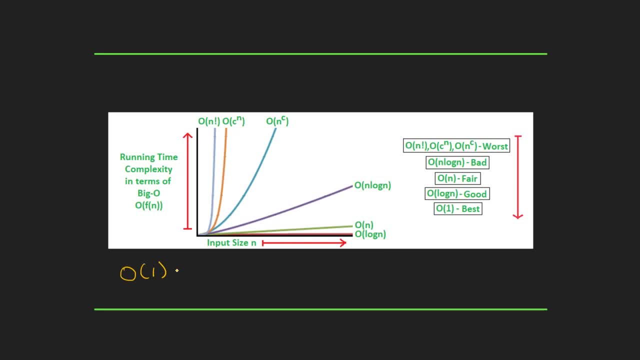 time complexities are a part of the quantity simultaneously, So, which is a greater time complexities will come out to be O Instead. if equals greater time complexity, this time complexity will be O. so the smallest and the best, Then we have O. 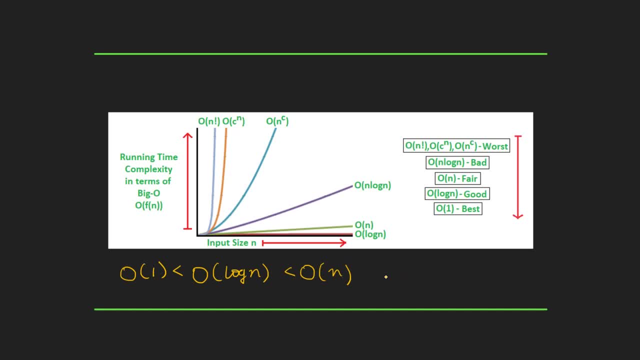 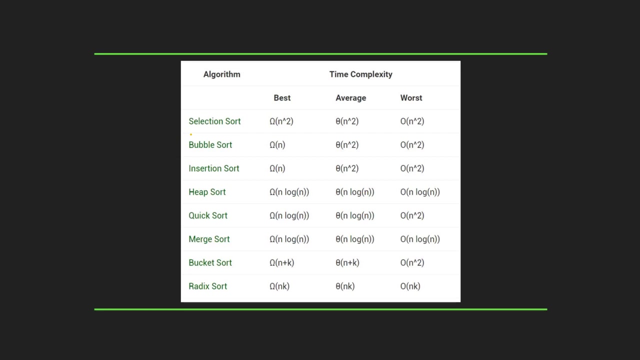 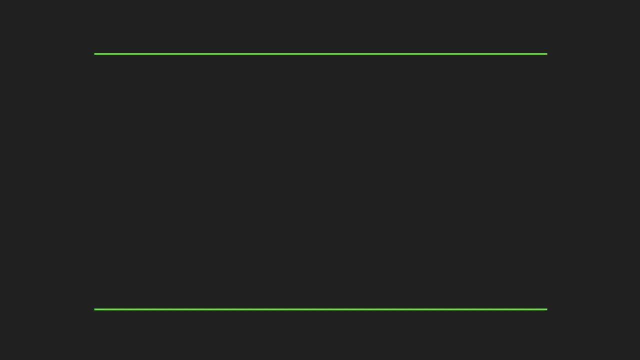 Then comes O, Then it is O, Then we have exponential time complexities And finally we have O, which is the worst. This is a chart of time complexity of various sorting algorithms. It is highly recommended to learn them by heart, as it comes very handy. Alright, so till now we have only talked about time complexity of a program. However, there 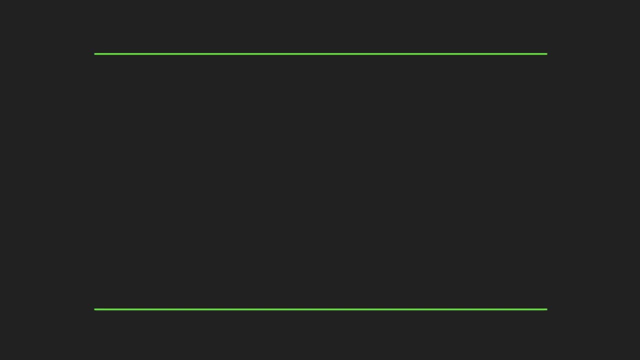 is another factor which affects the execution of a program, which is space. The space complexity of an algorithm quantifies the amount of space or memory taken by an algorithm to run as a function of the length of input. Let's quickly understand it with an example. Assuming that an integer takes 4 bytes of 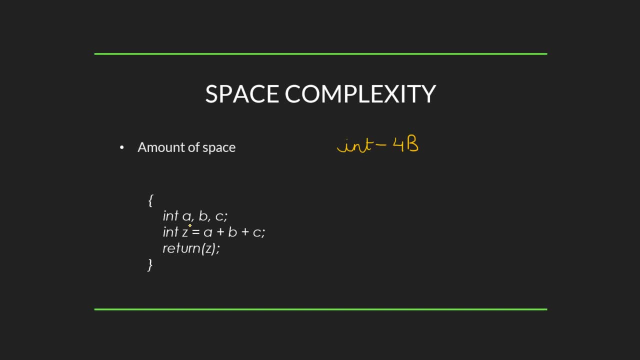 storage in memory. and in this piece of code we have 4 integers: a, b, c and z, So the total space will come out to be 4x4 plus 4.. This additional 4 is for the return statement. Hence this comes out to be 20 bytes. So this is a constant space running. 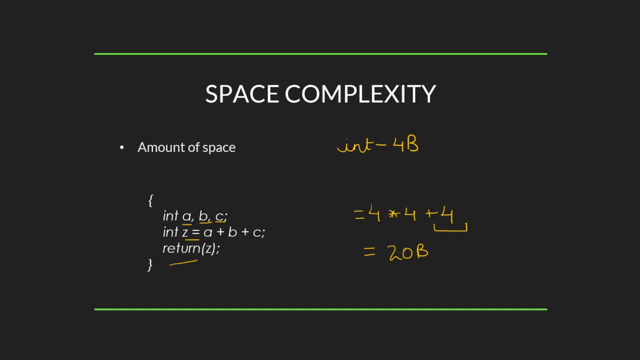 algorithm, There is usually a tradeoff between optimal memory use and runtime performance. In general for an algorithm, space efficiency and time efficiency reach at opposite ends and each point in between them has a certain time and space efficiency, So the more time efficiency.